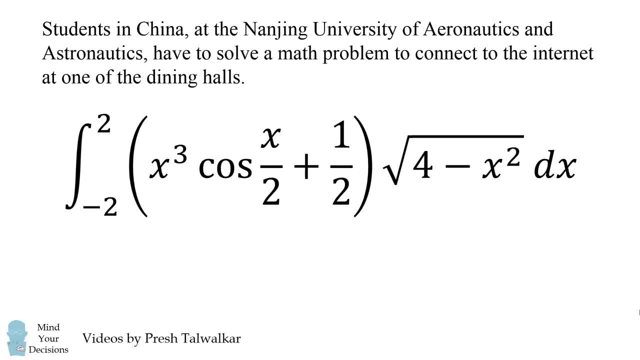 viral. It's the integral from negative two to two of the following quantity: We have x cubed times the cosine of x over two plus one half. We want that entire thing to be multiplied by the square root of four minus x. squared, The wi-fi password is the first eight digits. 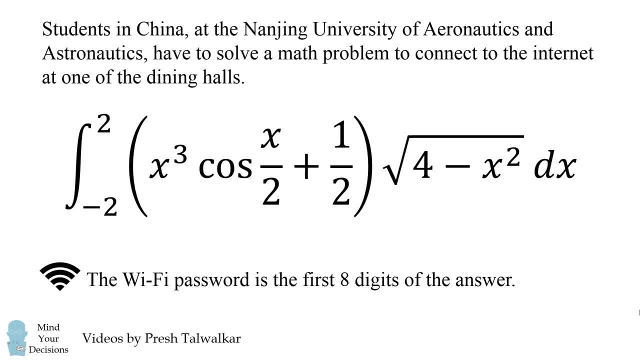 of the answer. Now. you can't use the internet to solve this problem because you're trying to get the wi-fi password and you're also not allowed to use calculators. You have to solve this using pencil and paper. Can you figure it out? Give this problem a try and when you're ready, 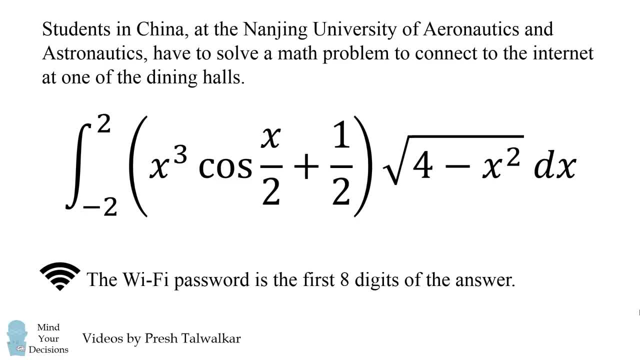 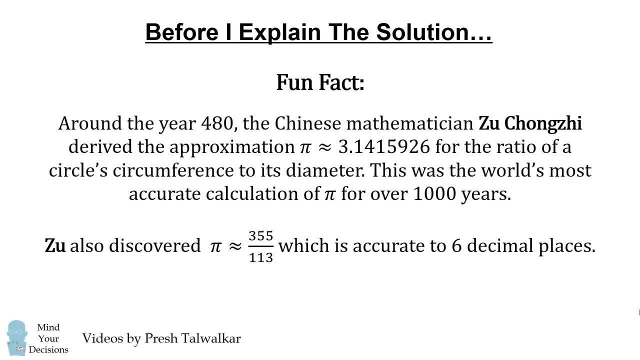 keep watching the video for a solution. Now, before I explain the solution, I just want to present a fun fact. Around the year 480, the Chinese mathematician Zhu Chengzi derived the approximation. pi is approximately equal to 3.1415926 for the ratio of a circle's circumference. 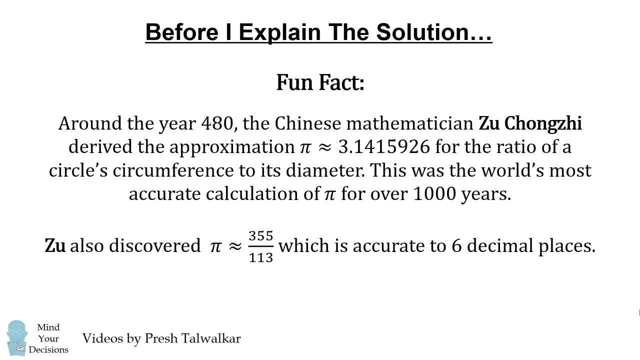 to its diameter. This was the world's most accurate calculation of pi for over 1,000 years. Zhu also discovered the rational approximation of 355 over 113, which is accurate to six decimal places. So, with that in mind, let's go ahead and solve this problem. How can we solve this integral? 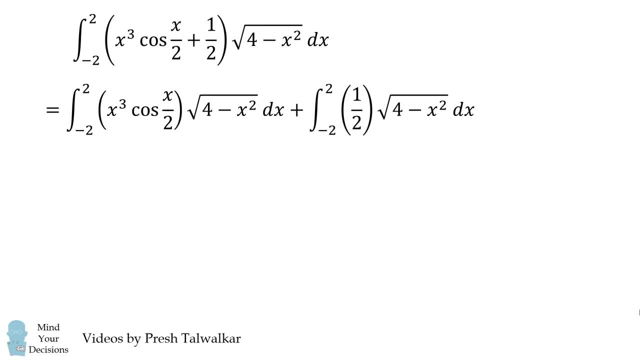 We'll first distribute what's in the parentheses, so we have two separate integrals. Now let's consider the integral on the left. We can evaluate it by considering even and odd functions. We can evaluate the integral on the left. We can evaluate it by considering even and odd functions. 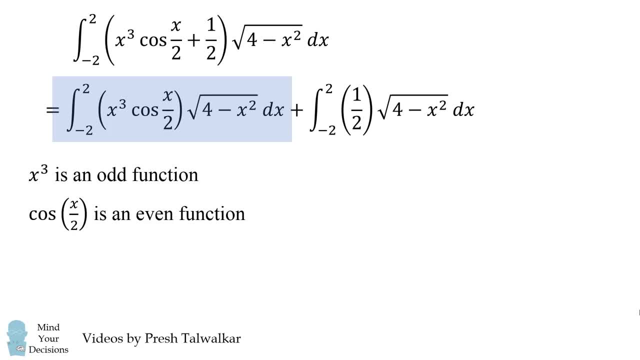 x cubed is an odd function, cosine of x over 2 is an even function and the square root of 4 minus x squared is an even function. We can put this all together to conclude: the product of these functions is also an odd function. Now recall the integral of an odd function over a symmetric interval. 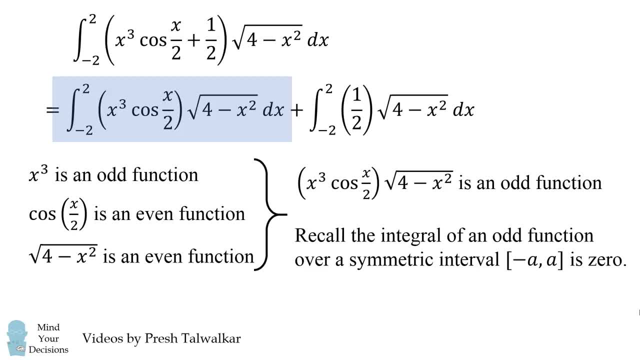 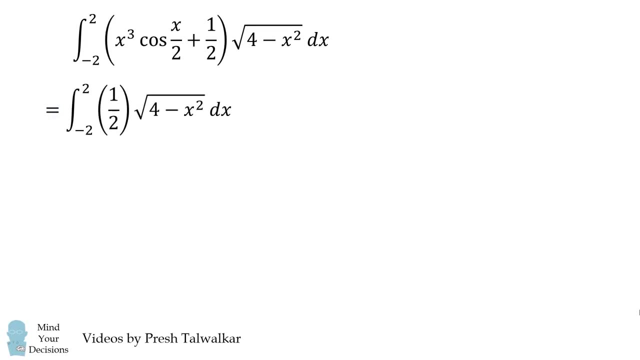 like negative a to a is identically zero. This means this entire integral vanishes and is equal to zero. So we've already simplified the problem tremendously. Now, how do we solve this integral? Remember that x squared plus y squared is equal to 4. 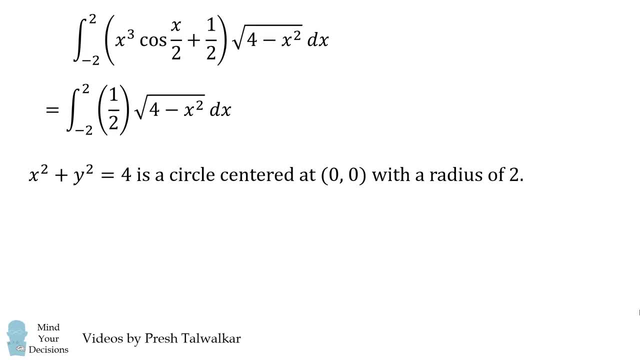 is the equation for a circle centered at 0,0 with the radius of 2.. So we can graph the square root of 4 minus x squared. So we can graph the square root of 4 minus x squared as being a semicircle. 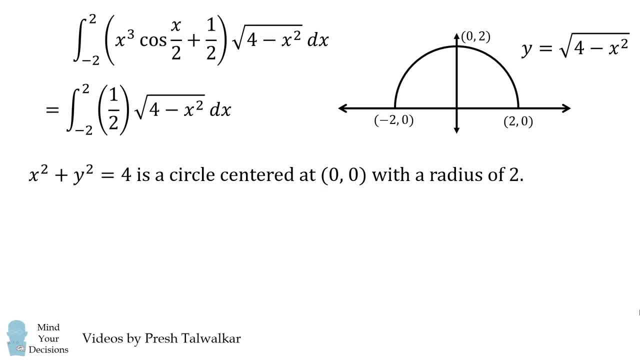 It'll have a radius of 2 and it'll just be in the positive y-axis. We want to calculate the area under here and then we want to take one half of the area, So the integral will be half the area of a semicircle with a radius of 2.. 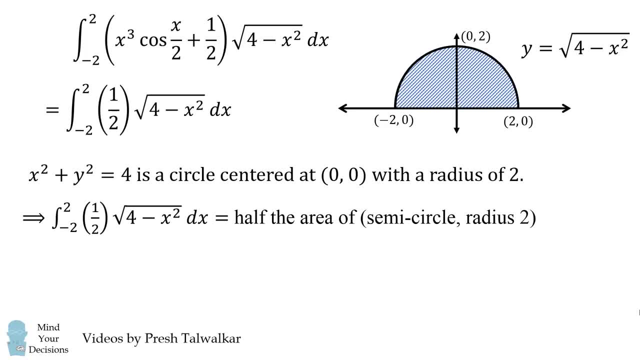 Pi r squared is the formula for the area of a circle. So we want one half pi r squared and then we want half of that. So we want one half of one half pi r squared, And this all simplifies to be pi. 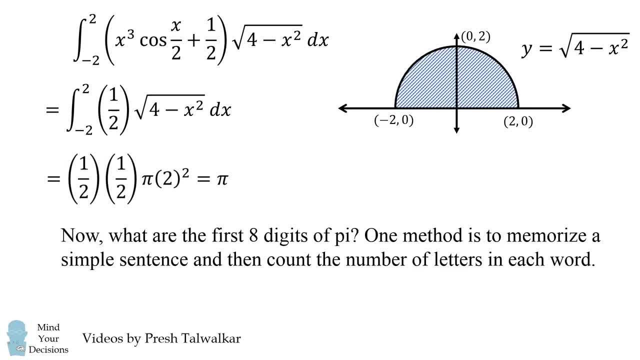 So that's the answer. But to get the wi-fi password we need to know the first eight digits of pi. How can you remember that? One method is to memorize a simple sentence and then count them. We count the number of letters in each word. 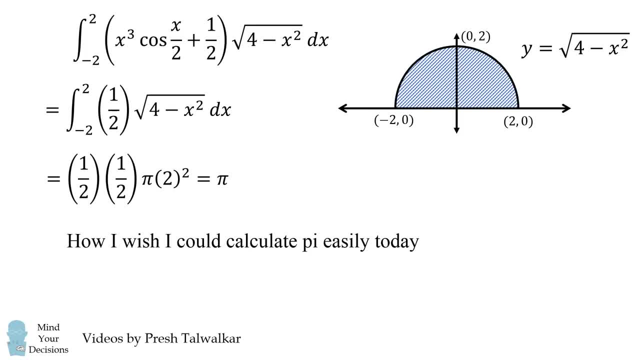 A sentence that I found online is the following: How I wish I could calculate pi easily today. Now we count the letters in each word, This will be 314159265.. The wi-fi password is the first eight digits, And that's our answer. 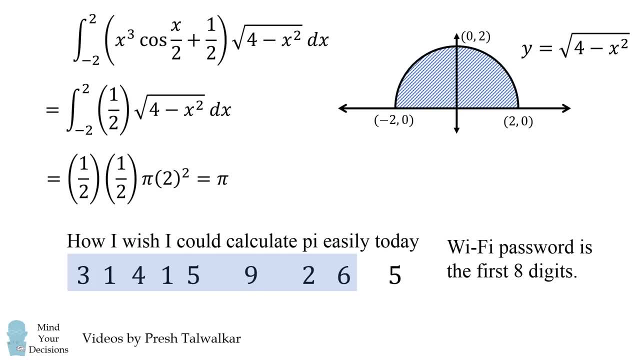 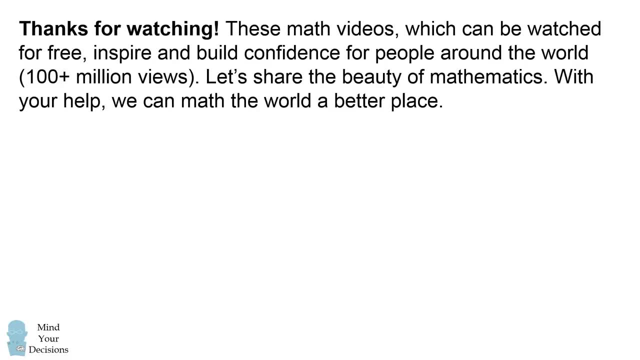 Did you figure it out? Thanks for watching this video. These math videos, which can be watched for free, inspire and build confidence for people around the world, And they already have over 100 million views. Let's share the beauty of mathematics. 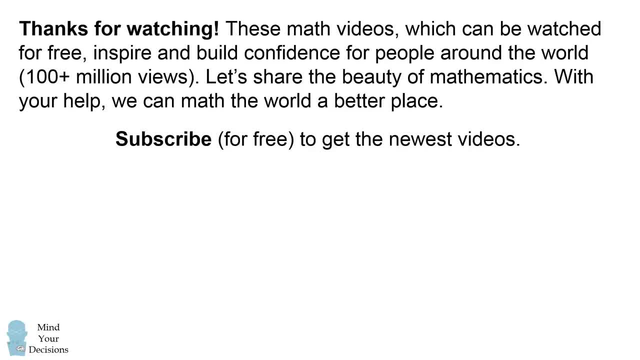 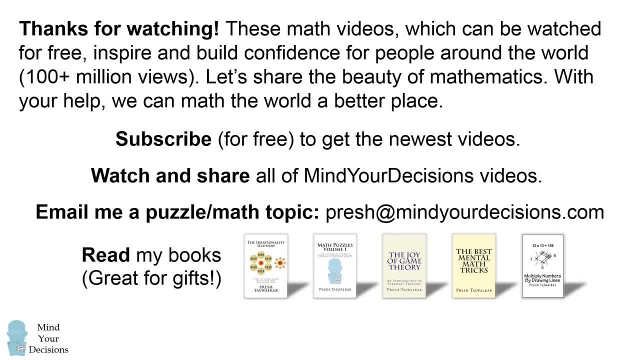 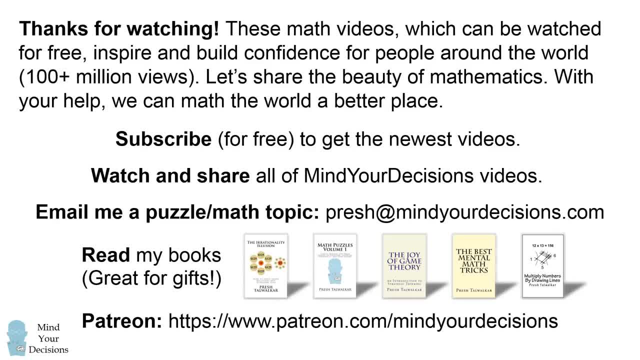 And you can support me on Patreon to earn exclusive rewards. Thanks for watching and thanks for your support.